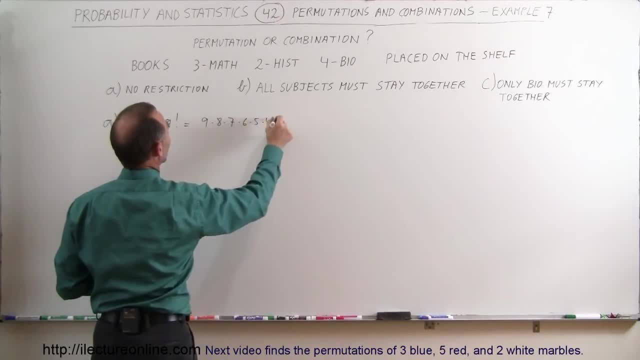 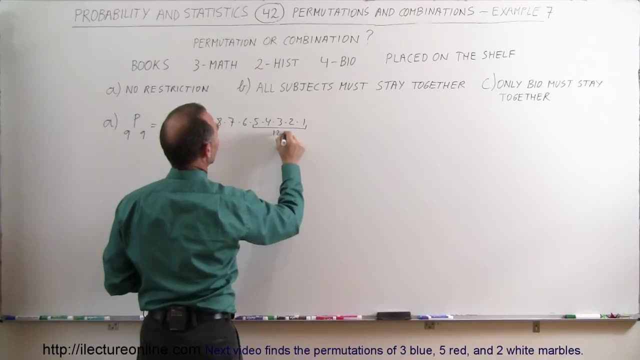 times eight times seven times six times, five times four times three times two times one. Well, we know that this here is equal to a hundred and fifty books. So we have nine books. So we have nine books. So 420 times six is equal to 720, and then, well, let's go ahead and 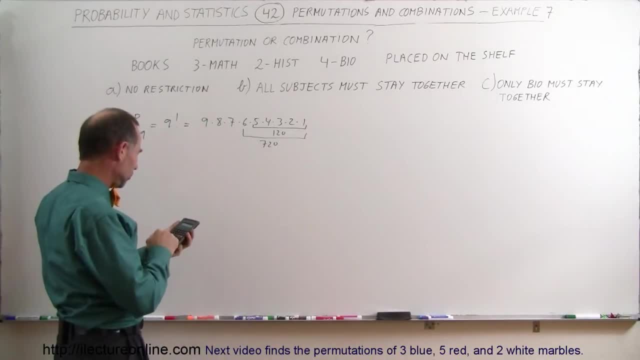 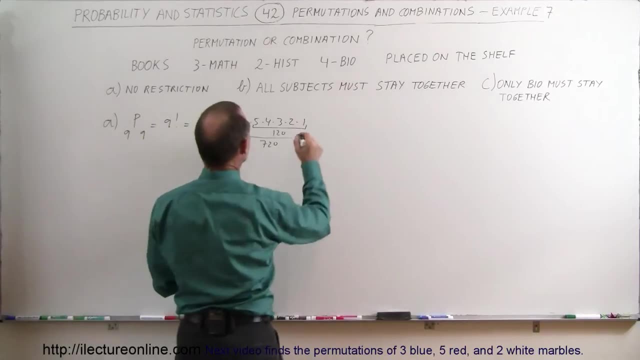 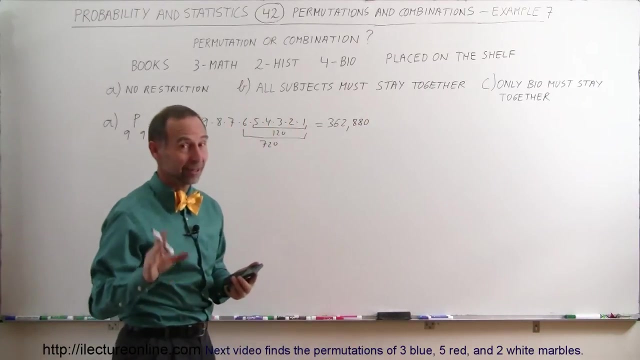 grab my calculator for the rest. So 720 times seven times eight times nine, and we get 360, 2, 880. combinations: 360: 2880.. I shouldn't say combinations, Permutations. Alright, Now for part B. all the subjects must stay together. 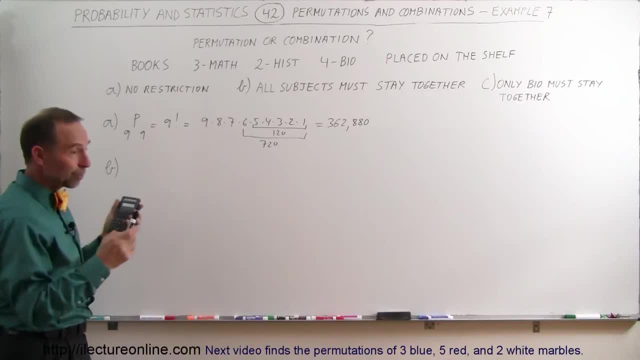 stay together, Which means that all the math books can be rearranged in a certain number of ways. All the history books can be rearranged in certain number ways, all the biology books can be rearranged in some other ways. And then, for each permutation of the math books, 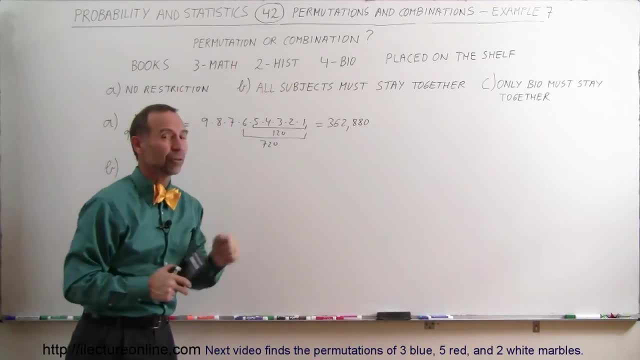 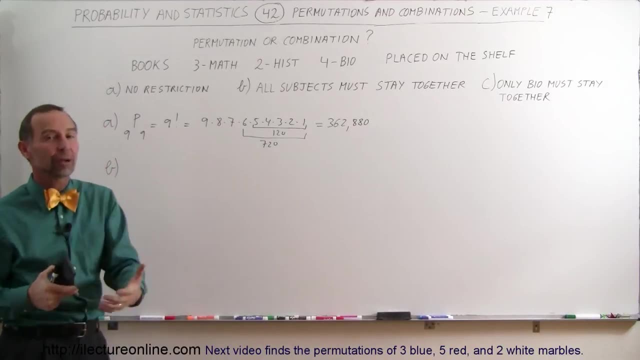 you can have so many permutations for the history books, so many permutations for the biology books, And then where the biology books and the history books are placed relatively to each other, that's another set of permutations. So the way that works then is: for part B we have three math books. 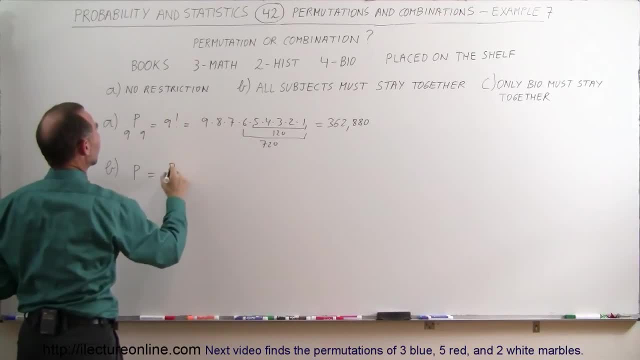 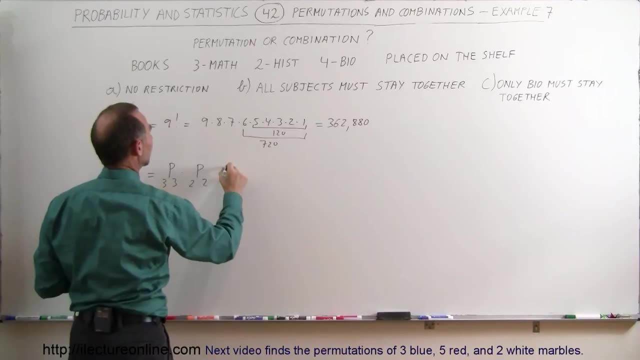 So for the math books. so the total permutations is equal to the permutations of the math books, which is 3 and 3, times the permutations of the history books, which is 2 and 2, times the permutations of the biology books 4 and 4.. 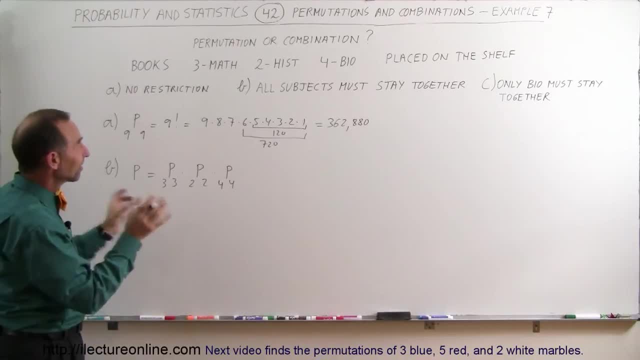 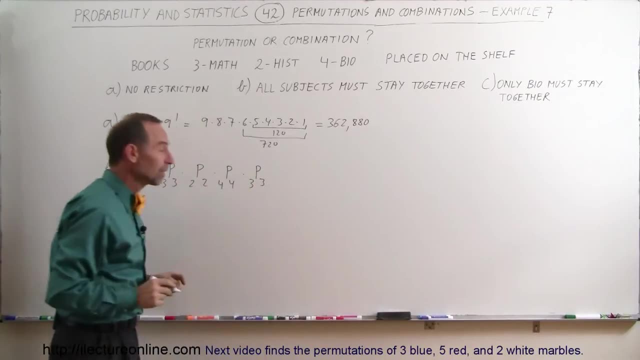 And now we have three sets, and the three sets can then be arranged in a number of ways, And so, therefore, times the permutations of three sets, which is 3 and 3, like that. Again, when these numbers are the same, that's the same as 3 factorial, 2 factorial, 4 factorial and 3 factorial. 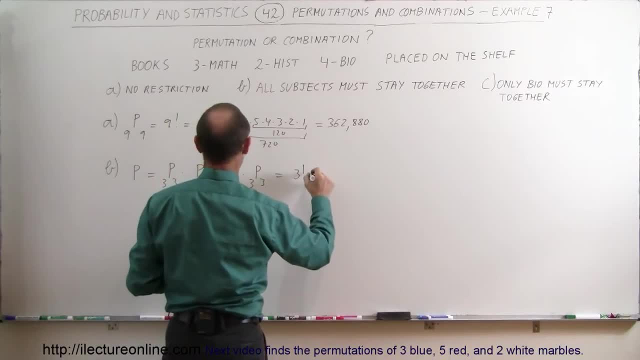 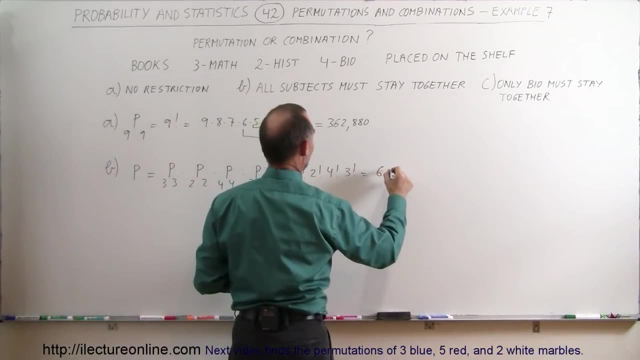 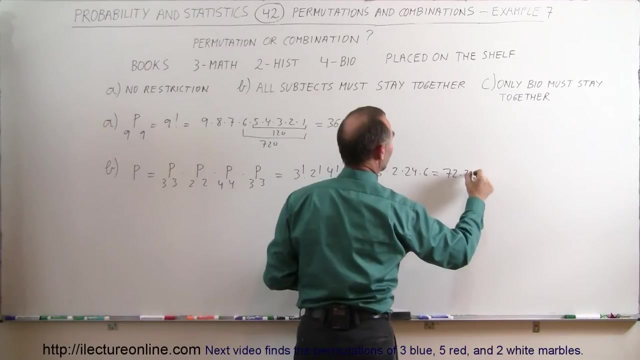 Or we can write this as: 3 factorial times 2. factorial times 4. factorial times 3 factorial, which is equal to 6 times 2 times 24 times 6,, which is equal to 36 times 2,, which is 72 times 24,. 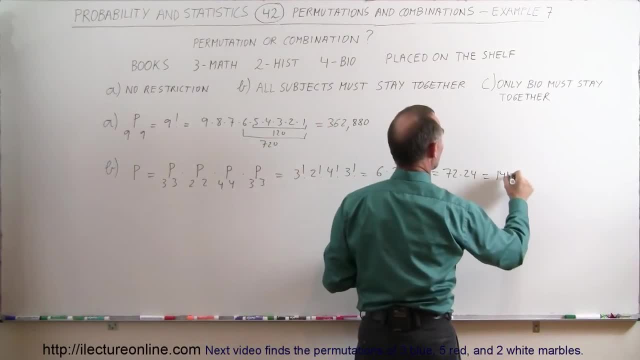 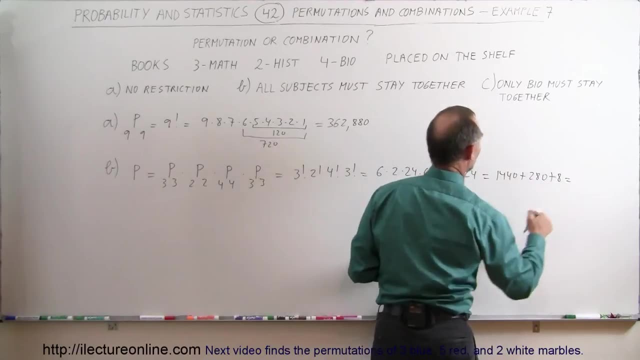 20 times 72,, which is 1440,, plus 4 times 70,, which is 280,, plus 4 times 2,, which is 8, and so that's equal to 16,, 17,, 20,, that's. 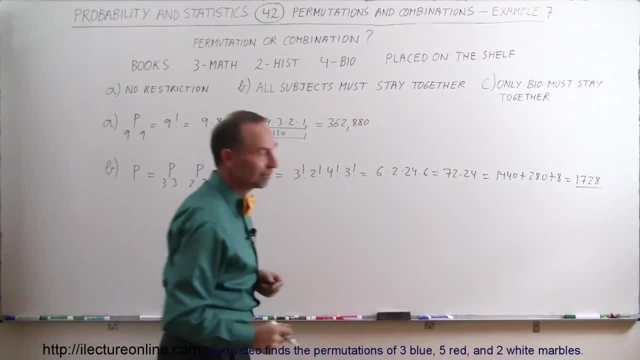 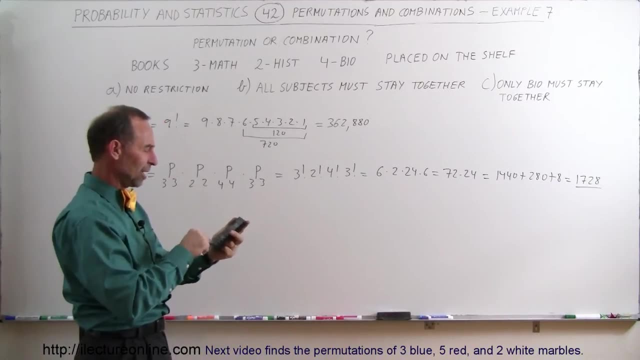 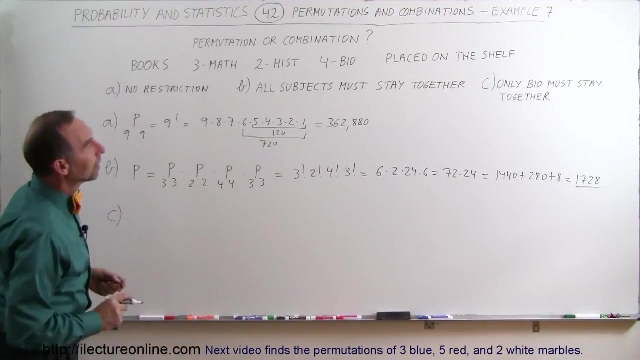 1,728 permutations. I hope that's correct. Why not go ahead and try it out with a calculator real quick to make sure I did it correct. 72 times 24 equals 17, 28.. That is correct. Finally, for part C, only biology books must stay together. All right, let's see then. We have three. 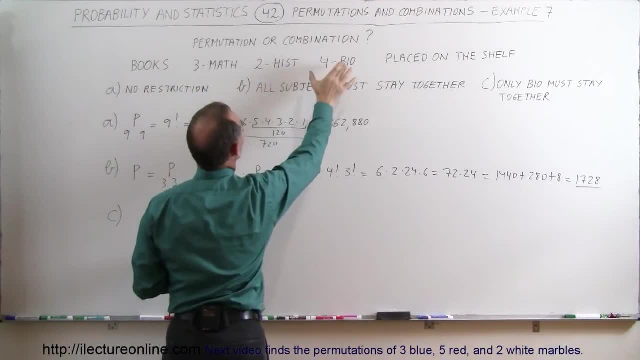 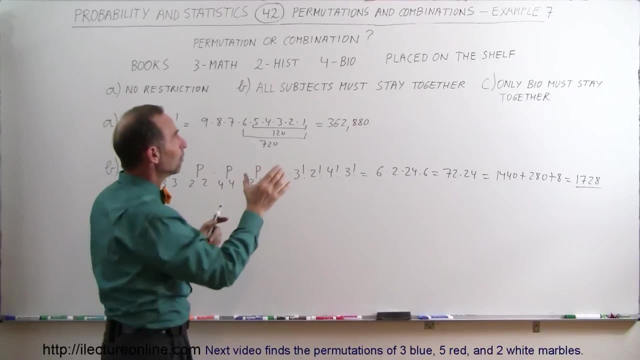 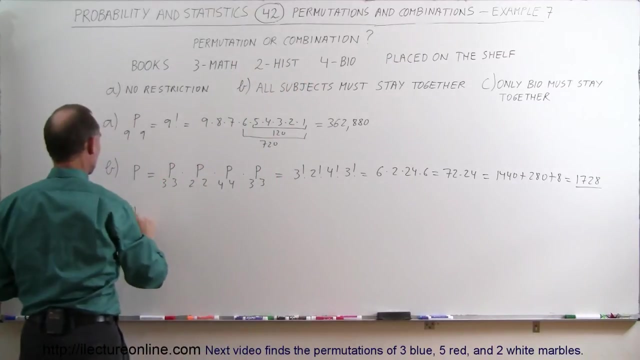 math books, two history books and four biology books. but if those stay together, what we can then assume for the time being is: let's keep them all together in one order and think of this as one single book. and so we have 1 times this times this, so that means the number of permutations is 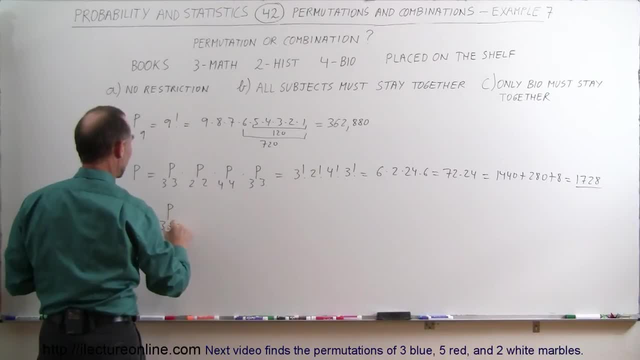 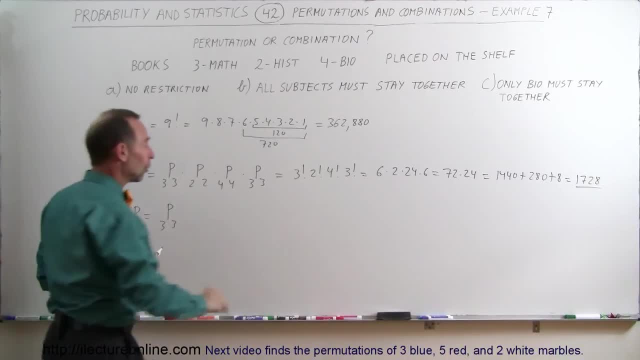 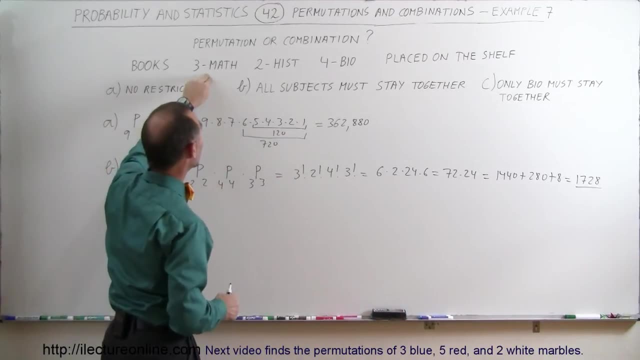 for the history books. well, wait a minute, they don't need to stay together. so, actually, what we can think about is this way. That's a better way to think about it and actually the correct way. Notice that we have three math books and two history books, and they can be arranged any. 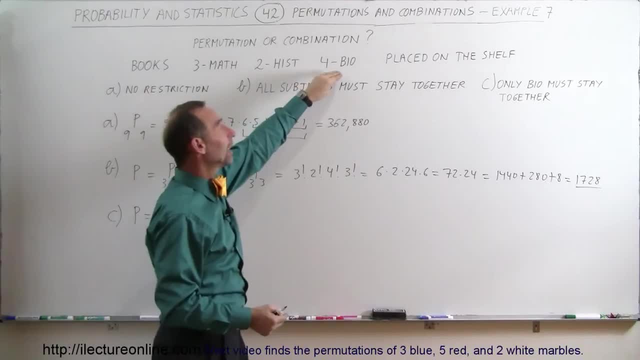 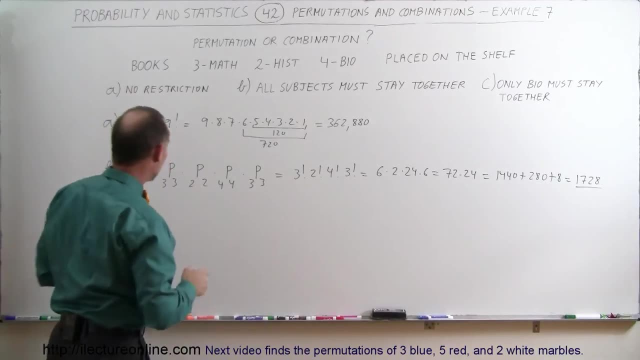 which way we want. so it's actually like five books and then those four biology books put together. think of this as one book. then we have a total of six books. that can be arranged in any which way we want. Therefore, it'll be the number of books that we want, and then we have. 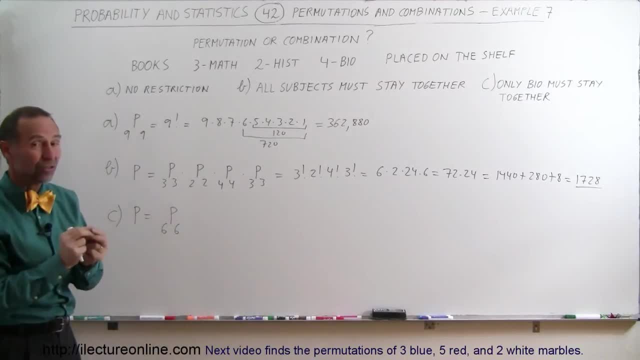 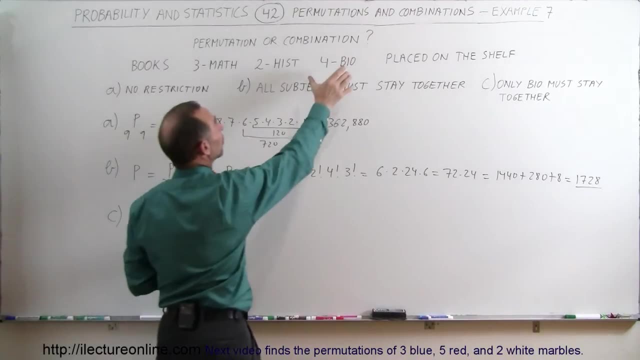 permutations of six, and six means three, math, two history, and all the biology books put together is as if we had six separate books. but then we have to realize that the biology books can also be arranged within themselves in a number of ways, and so we have to multiply that. 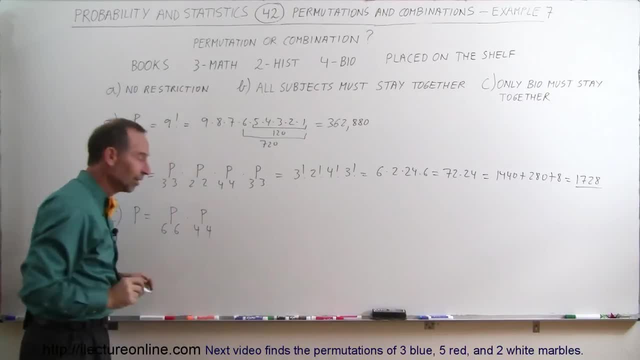 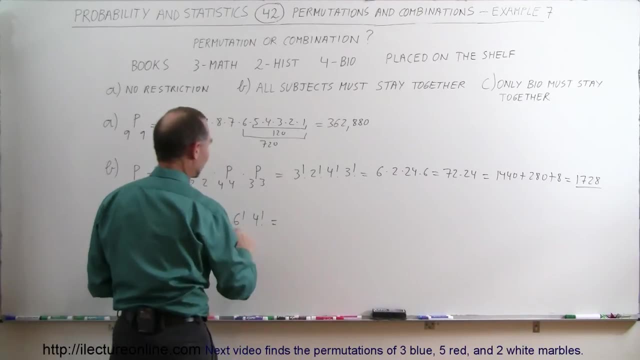 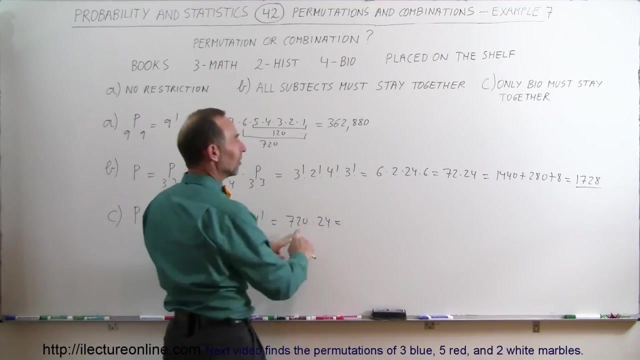 times the permutations with four books and four spaces, and so this then becomes equal to six factorial times four factorial, and so six factorial would be equal to 720. four factorial factorial is equal to 24, so this would be 720 times 24,. that would be the same as that with 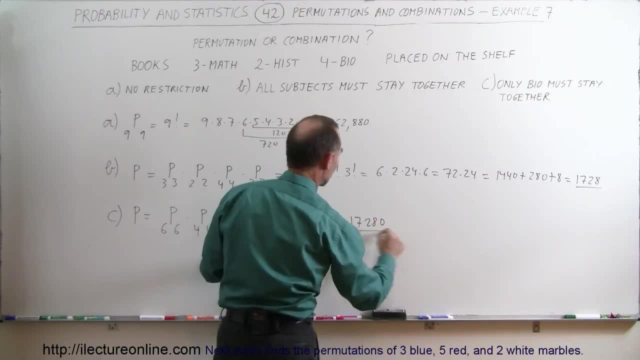 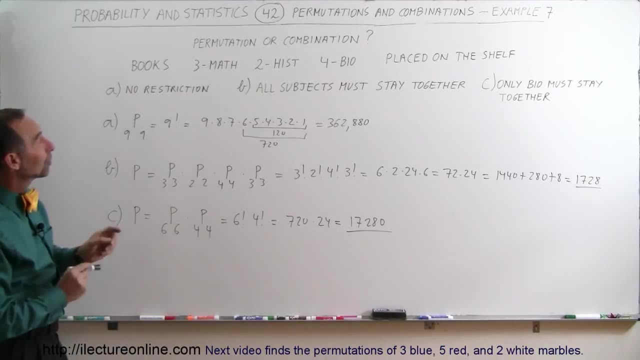 another zero, 17280, so it would be 17,280 different permutations when you have, let's see here, three math books, two history books, which can be arranged any way. you want four biology books, which need to stay together. That's how we do that.